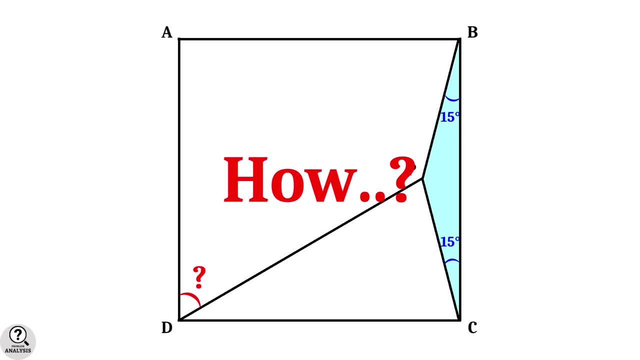 Now just think: How can we find that angle? From the figure you can calculate some more angles. Angle BPC will be 150 degree Because, as you know, sum of angles in a triangle is always 180 degree. Then angle, ABP and angle. 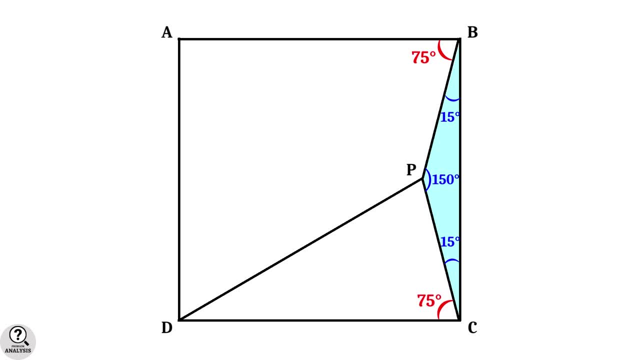 DCP are 75 degree each, Because each angle on a square is 90 degree And also, by the same reason, angle A equal to 90 degree. That's all. No more angles we can find using simple calculations. For now, let us all try video. even if we use trigonometry, it is very difficult, But 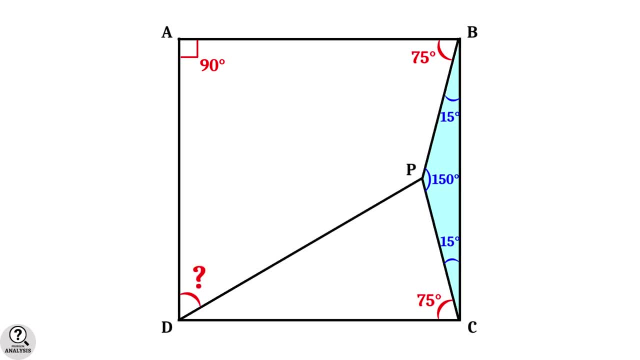 still we have to find the angle ADP. So there should be some trick, and I am going to explain what that trick is. It is simple but powerful. Let's see: Take a copy of the triangle BPC and place it on. 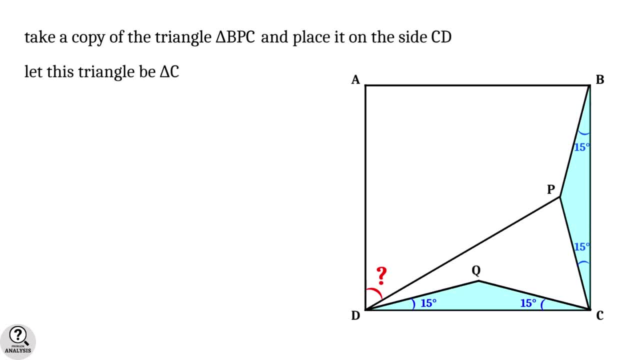 the bottom side of the square. Let this triangle be triangle CQD. Now there is another triangle, CPQ I. In this triangle, angle C, equal to 16 degree, 90 degree minus 2 times 15 degree, that's equal to 60 degree. Also, the sides CQ. 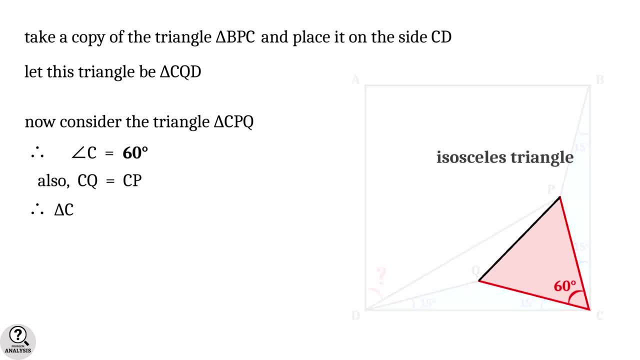 equal to CP. therefore, triangle CPQ is an isosceles triangle. Now, by the property of isosceles triangles, the angles opposite to equal sides are also equal, which implies here angle P and angle Q are equal and their value is 180 degree minus 60 degree, whole divided by 2, which is equal to 60 degree. What does 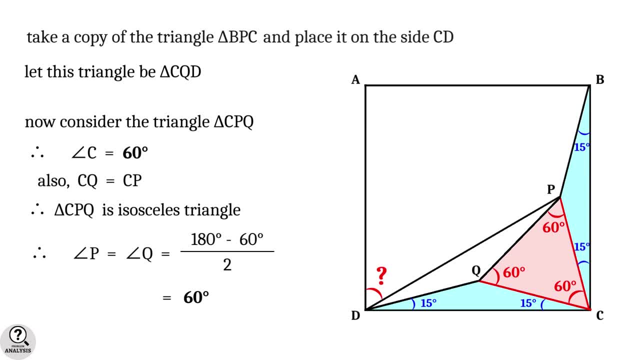 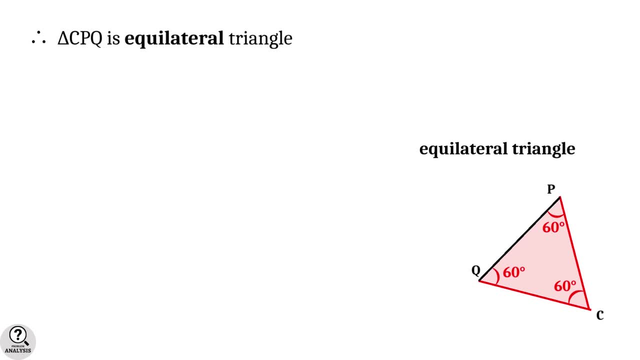 it mean All the angles are equal to 60 degree. therefore, triangle CPQ is an equilateral triangle and therefore, by the property of equilateral triangles, all the sides are also equal. Now consider the triangle CQD. Since the sum of angles in a triangle is always 180 degree, then angle Q. 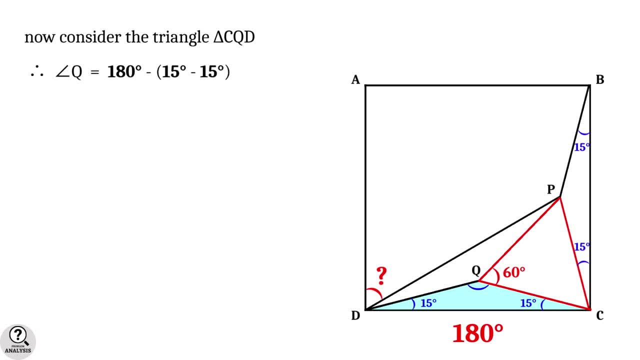 will be 180 degree minus 2 times 15 degree, which is equal to 150 degree, and therefore angle DQP equal to 360 degree minus 150 degree plus 60 degree, which is equal to again 150 degree. Now everything is going to be very clear. Consider the two triangles CQD and PQD. Observe that.